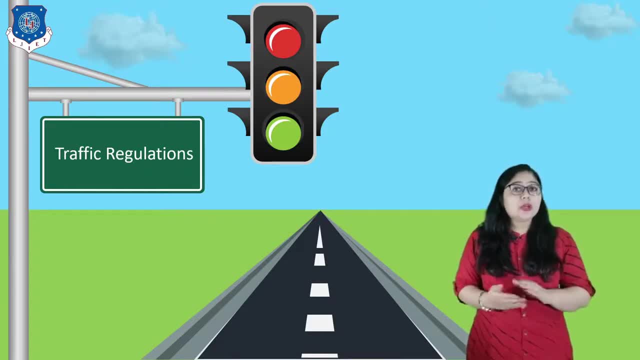 Some traffic rules and regulations are like: do not drink and drive and users of road should avoid to alcohol before and while driving. In order to have safe traffic operations on road, it is essential to impose adequate traffic regulations. So basically it is divided into three parts. 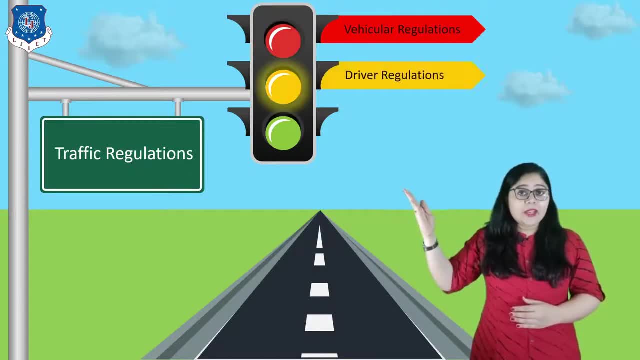 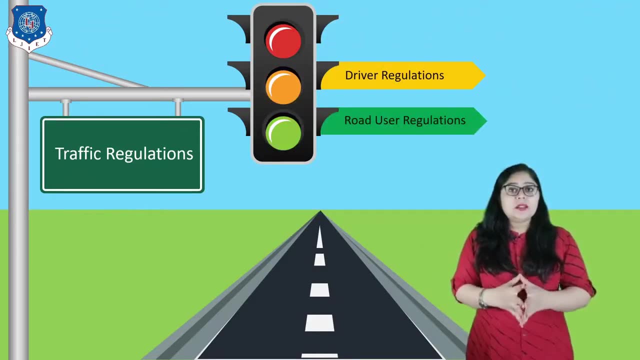 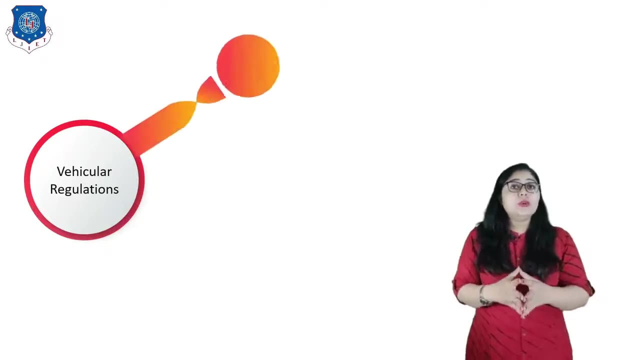 First is vehicular regulation, second is driver regulation and third is the road user regulations. So first let us discuss what are the vehicular regulations are. So, to understand it, first we have to do registration of any vehicle, which is known as RC book. 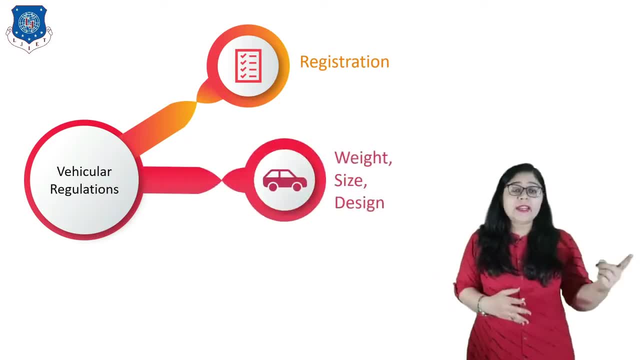 Then after we have to classify vehicles according to their weight, size and design, Say for example, say, for example, I talk about a four-wheeler, then it can be separated as a heavy truck. also, Even size and design of normal car and a heavy truck is so different, So we have to keep all the constraints. 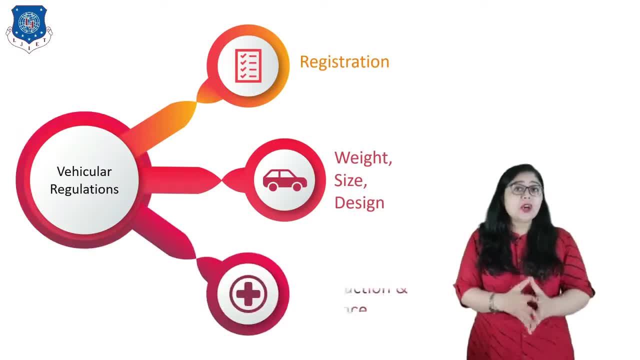 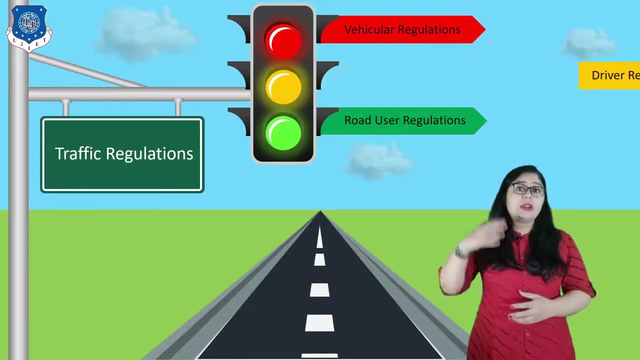 in mind. Lastly, we have basic knowledge of construction of any vehicle. Even insurance of any vehicle plays a key role, while we want to claim it. So it is all about this vehicular regulation. Now let us discuss our second part, which is driver regulation. So, driver regulation. 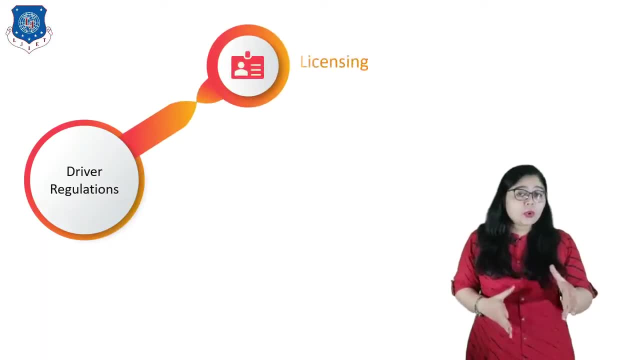 can be done by licensing. As we know, a person must give driving test to get license, where the driving skills are tested, and without license, driving any vehicle is a crime. Next is physical fitness and age of driver that matters. Say, for example, we prefer experienced 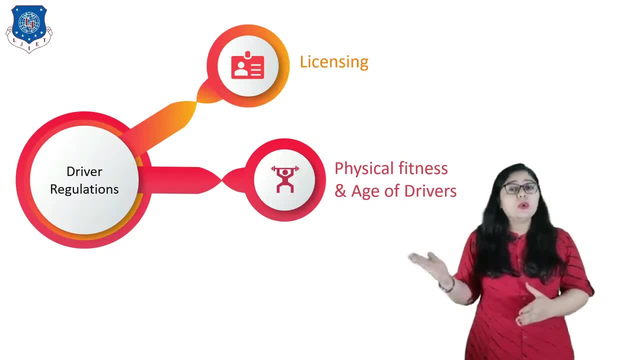 drivers. We prefer experienced drivers. We prefer experienced drivers. We prefer experienced driver who is not too young and also not too old, Because with age, psychological condition as well as the quick decision taking skill reduces, While in younger stage with aggression. 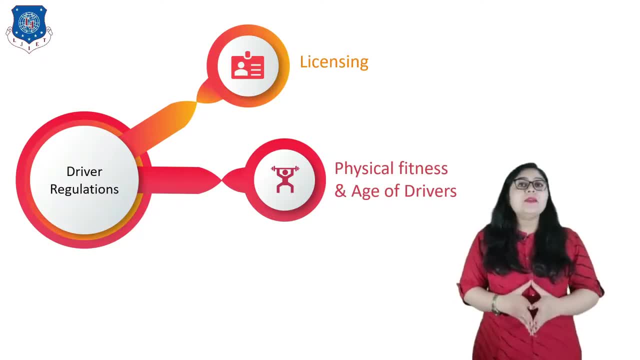 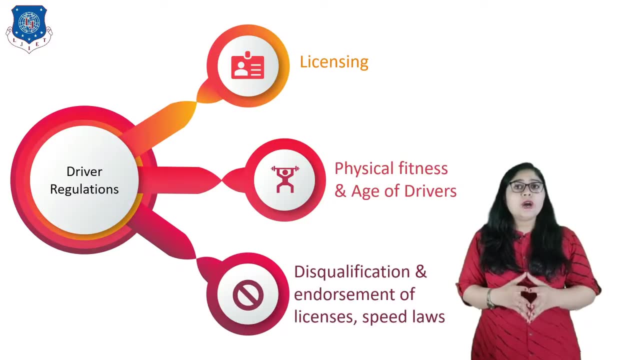 chances of accident are still there. And lastly, we will discuss about disqualification and endorsement of licenses and speed laws. Mortaring offenses can incur fines and endorsements. An endorsement on your driving license means that you have been given points which will remain on your license until they expire, Depending on the type of offense committed. 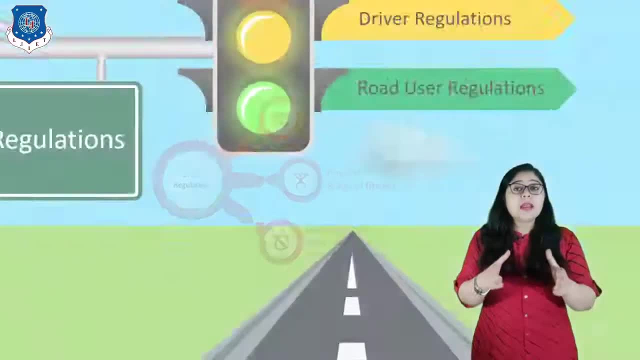 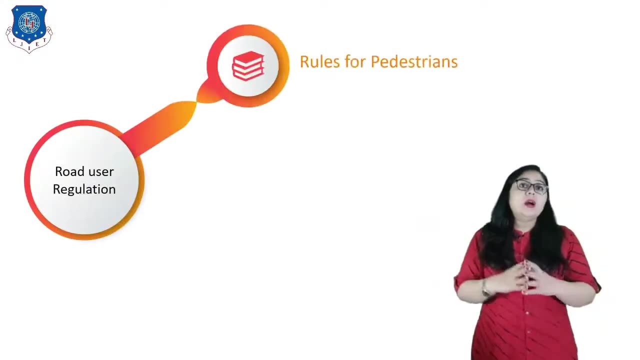 this is usually 4 or 11 years. Now. next is road user. Here we have to also think for pedestrians: Crossroads: where there pedestrians are crossing, Always walk on footpath. where there is no footpath, Walk in the right side margin of the road so that you can see the traffic. 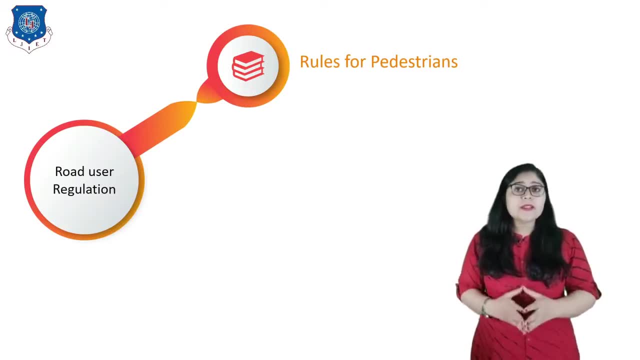 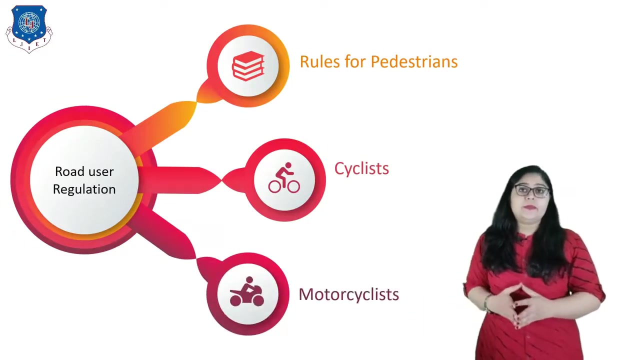 coming in the opposite direction. Next is about cyclist. We should provide separate route for cyclist to ensure their safety and comfort on the road. Last but not least, we should provide facility to motorcyclist. Now let us move to our second topic for today's lecture, which is all about 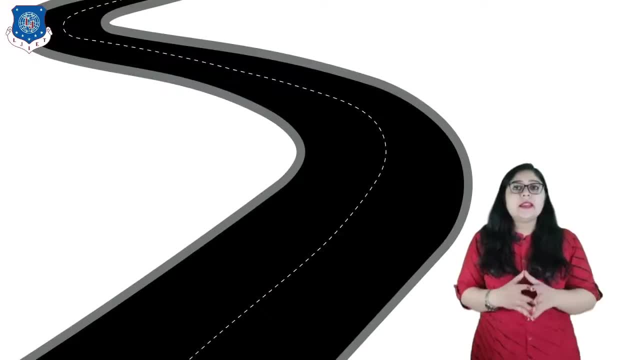 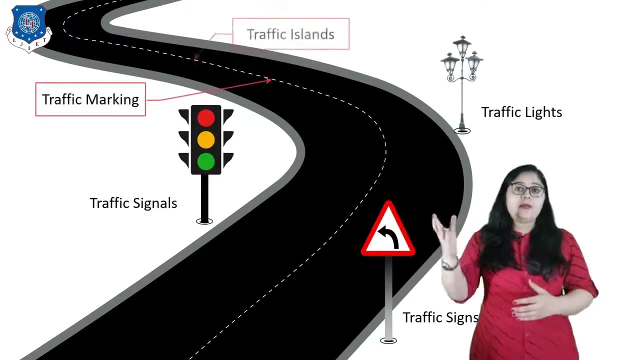 traffic control devices. The various aids and devices used to control, regulate and guide traffic may be called as traffic control devices. Broadly, these fall into five categories. First is traffic signs, then traffic signal, traffic lights, traffic marking and traffic islands. Now let us discuss traffic signs first. 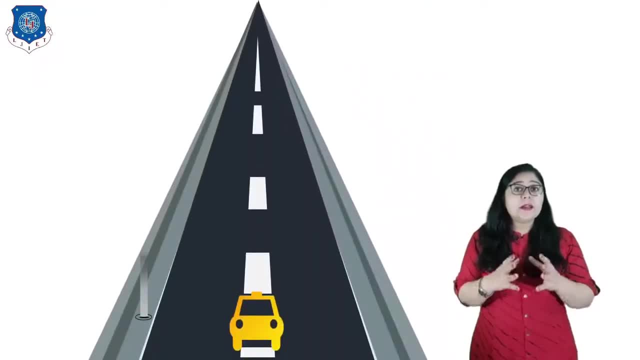 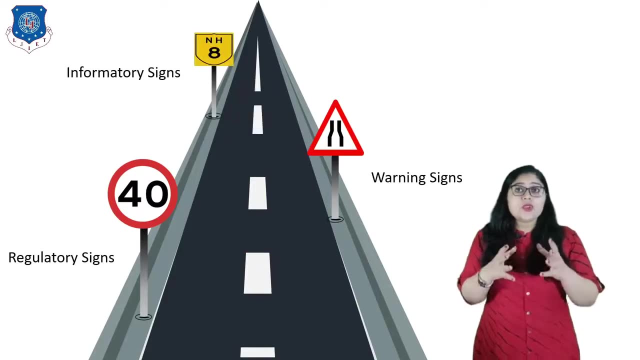 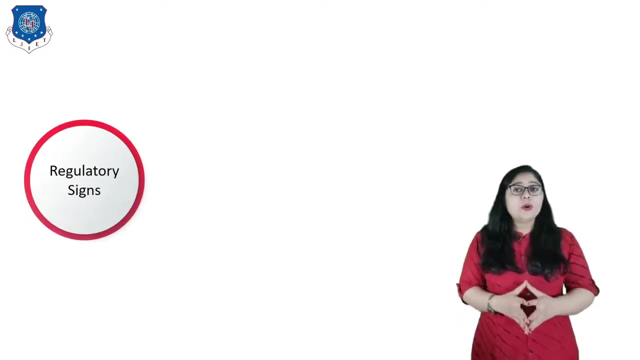 So basically it is classified as regulatory signs, warning signs and the informatory signs. So let us discuss regulatory signs first. Regulatory signs are meant to inform the road users of certain laws, regulations and prohibitions. It is further classified into two types, where the first is directional road signs and second is the 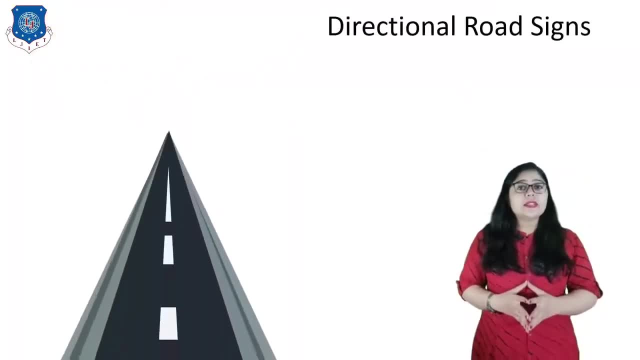 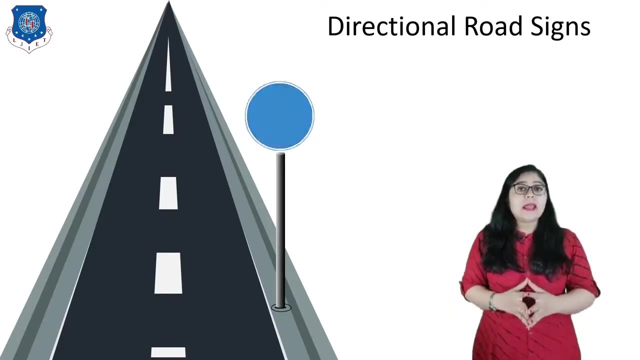 prohibitory signs Here. directional road signs have blue background and white background. Different types of regulatory road signs are like: compulsory turn left. compulsory turn right. compulsory turn left ahead. compulsory turn right ahead. compulsory keep right. compulsory keep left and compulsory: proceed ahead. Now let us discuss prohibitory signs. They have basically white. 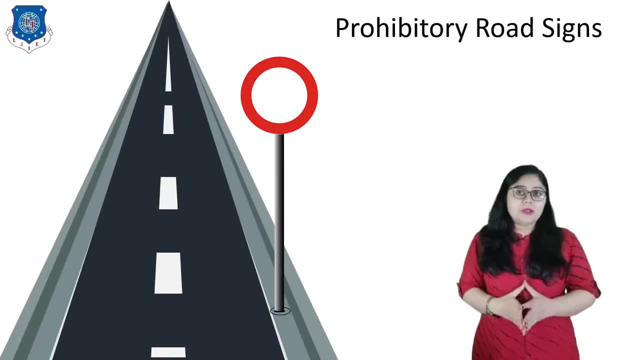 background, red border and black symbols. Now let us discuss the red border and black symbols. So different types of prohibitory signs are like: no parking, no entry, no left turn, no right turn, no overtaking, no stopping, no u-turn, no horn speed limit and the width limit. But 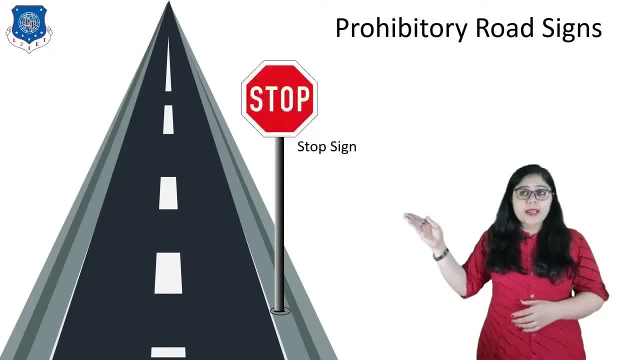 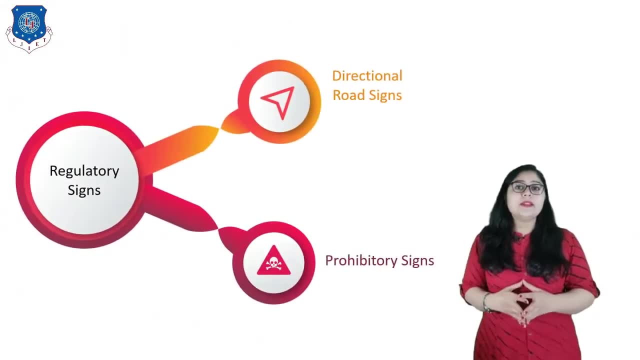 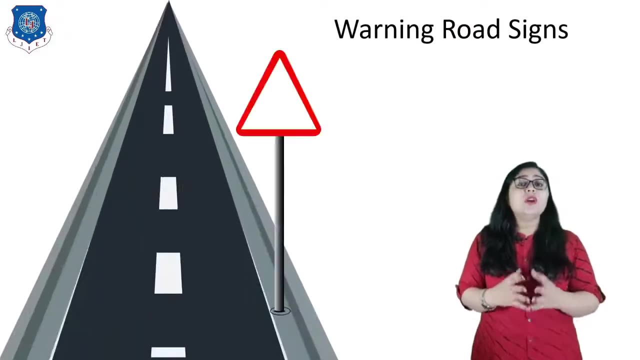 here are few different cases, like stop sign and give way, which has their unique symbols. That's all about regulatory signs. Now let's move to the next topic: warning signs. So warning signs are used to warn the road user of certain hazardous conditions that exist on or 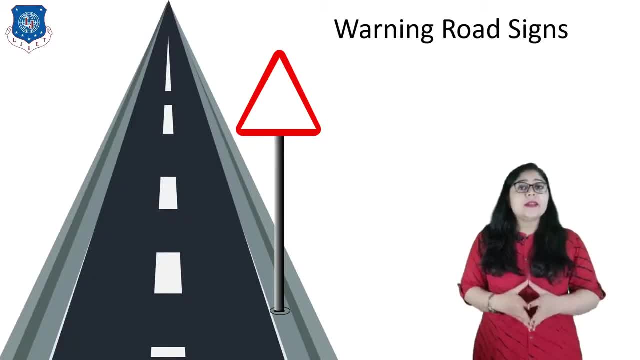 adjacent to the roadway. Warning signs are to great help in ensuring safety of traffic. They have white background, red border and black symbols. Signs are to be located at sufficient distances are 120, 90, 60 and 40 meter respectively, on national highway or state highway or major. 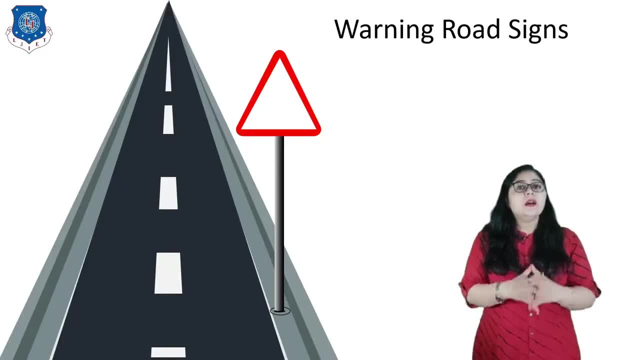 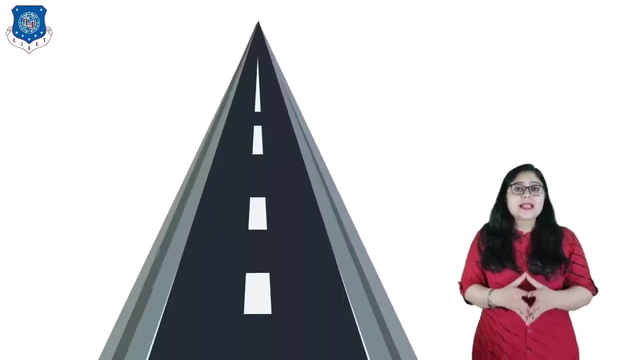 district road or ordinary district road and village road. Different types of warning signs are like left hand curve, then after right hand curve, narrow bridge, man at work, uneven road, narrow road, roundabout, T-intersection, side road, right and cross road. So now last type of traffic sign is: 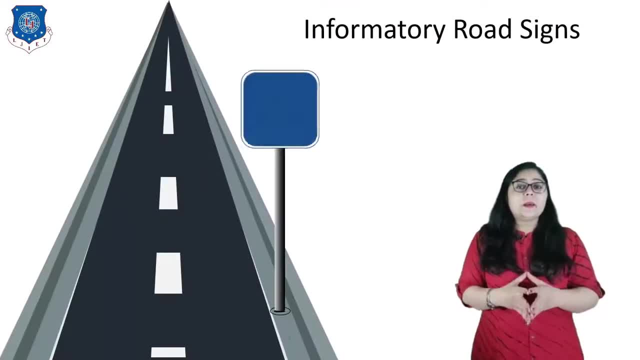 informatory road signs. These signs are meant to provide information on direction, destination, road side facility, etc. to the road user. 20 00 00 00 00 00. This road signs helps a driver in saving time reaching destination while looking around. 21 00 00 00. 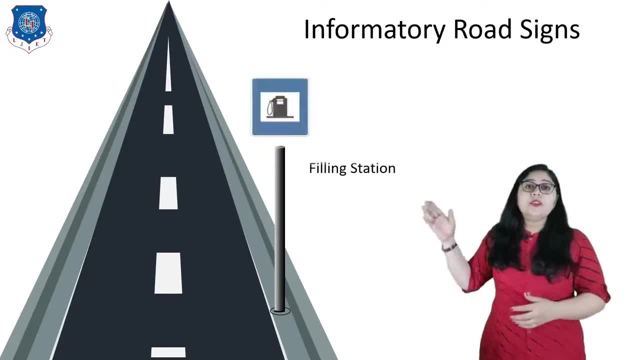 These signs are normally blue in colour. 23 00 00 00. Different types of informatory signs are: filling station, restaurant, hotel, parking, first aid, post, refreshment, hospital. 24 00 00 00 00. 24 00 00 00, 20 00 00 むむ, But they can also be chosen to unlock thewehre system in Santa Cruz. 21 00 00 00 00 00. Pareline point or spaces can be assigned on the road at any time. different issues can be. identified during the truck. it is no law of gravity that the driver is the driver. They can be a person when driving. 22 Ah. 21 00 00 00 00 00 000. However, μα одно road used as traffic and rent can be connected to the road. 24 00 00 00 00 00 00. 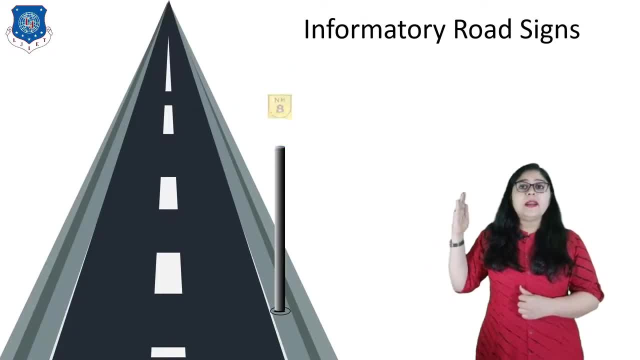 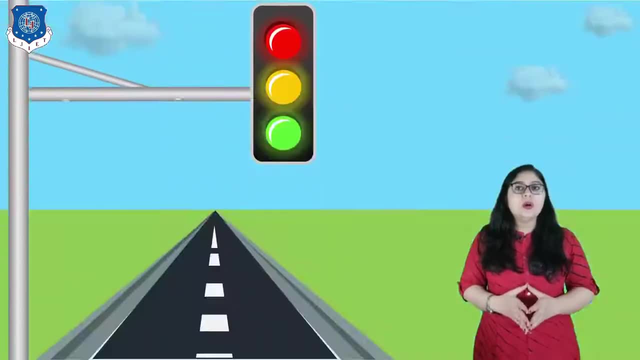 bus stop, road maker sign and road junction approach. Now let's discuss next topic: traffic signals. So a traffic signal is used as an instructing device that indicates the road user to act according to the displayed sign. Following the traffic signal ensure road safety. 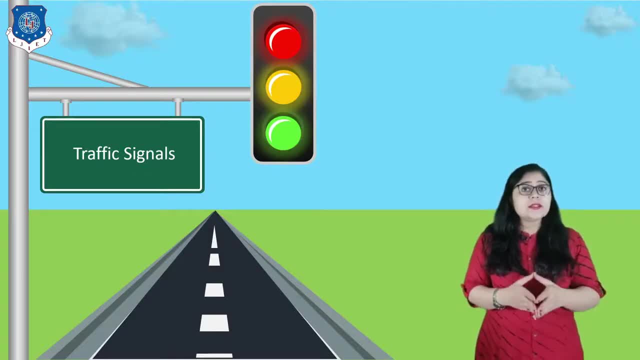 and to make things simple to understand, these signals have been using a universal color code. There are various type of traffic signals are used. First is fixed time signal. These signals are set to repeat regularly a cycle of red, amber, yellow and green lights. 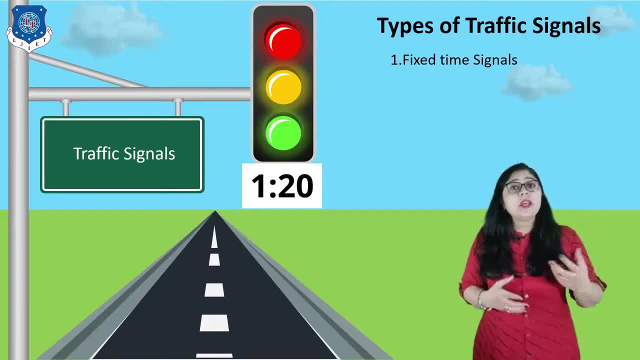 Depending upon the traffic intensities, the timing of each phase of the cycle is predetermined. Fixed time signals are the simplest type of automatic signals that can be used to detect traffic signals which are electrically operated. But the drawback of this signal is that the cycle 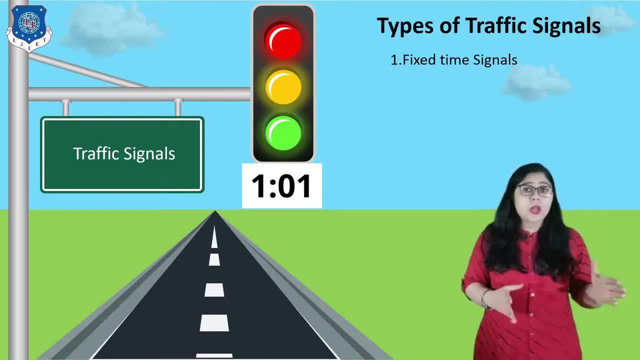 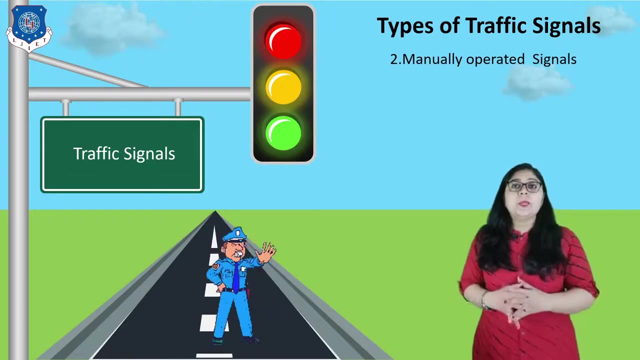 of red, yellow and green goes on, irrespective whether on any road there is any traffic or not. Also, traffic in the heavy stream has to stop at end phase. Second type is manually operated system. In this system or in this type of signal, the traffic police watches the traffic demand. 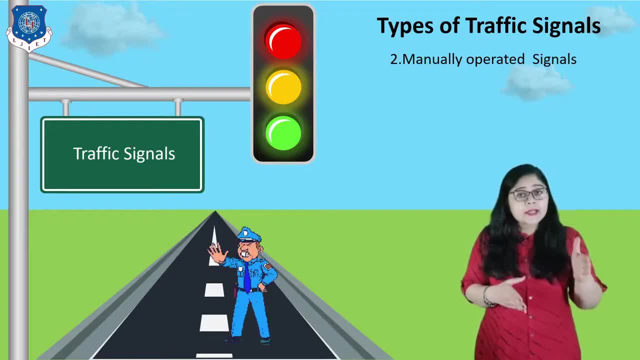 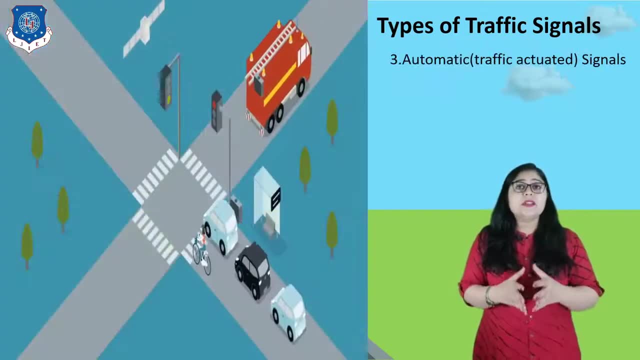 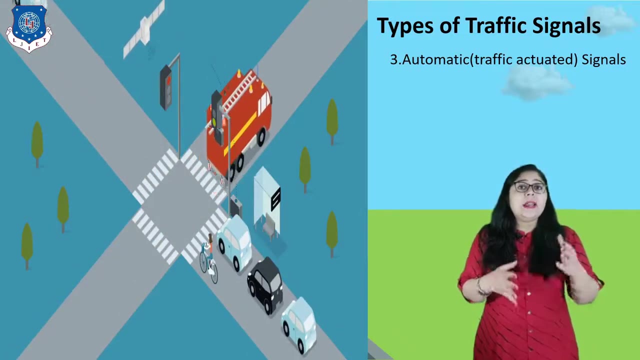 for a suitable point during the peak hour at the intersections and varies the timing of these phases and cycle accordingly. Third type is traffic actuated or the automatic signals. In these signals, the timing of the phase and cycle are changed according to the traffic demand. 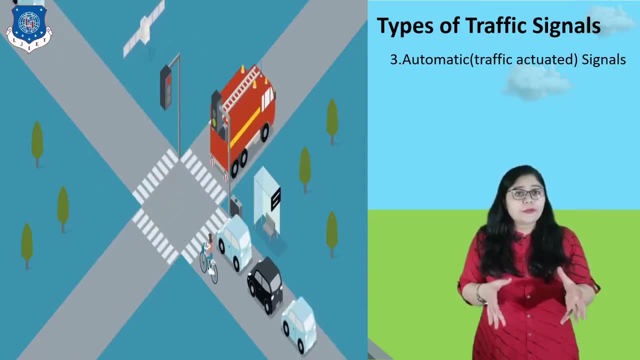 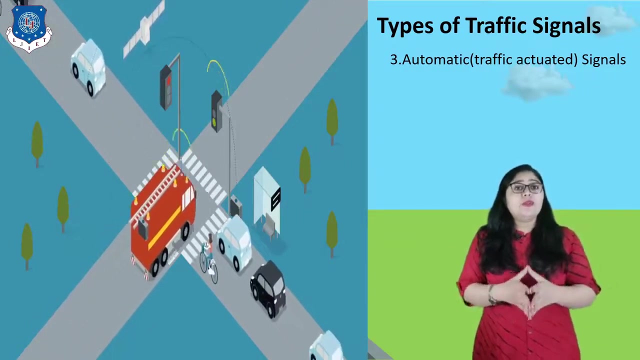 In semi-actuated signal, the normal green phase of a traffic stream may be changed according to the traffic demand. The traffic movement of the traffic signal may be extended upto a certain period of time for allowing the vehicles to clear off the intersections, While in fully actuated signals, computers assign the right of way. 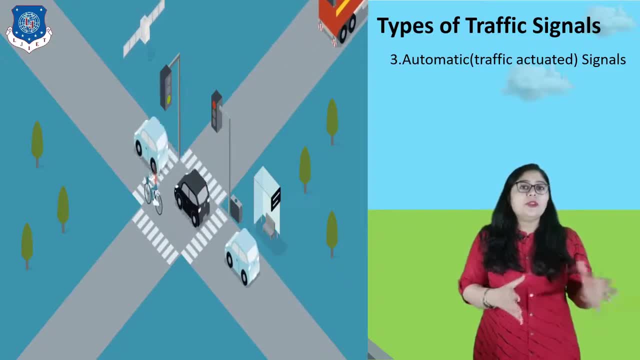 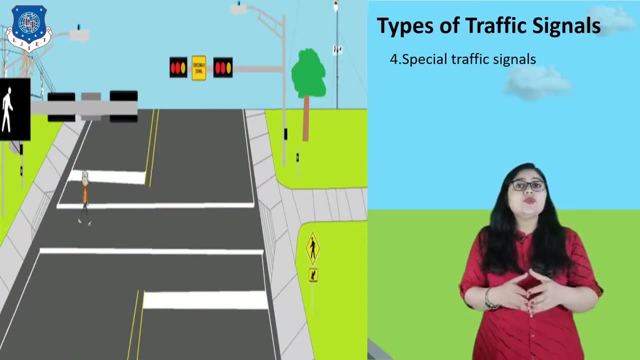 for the traffic movement on the turn basis of traffic flow demand. Fourth type is spatial traffic signals. These signals are used to warn the traffic. When there is a red flashing signal, the drivers of the vehicle must stop before entering the nearest crosswalk, at the intersection or at a stop line where marked. 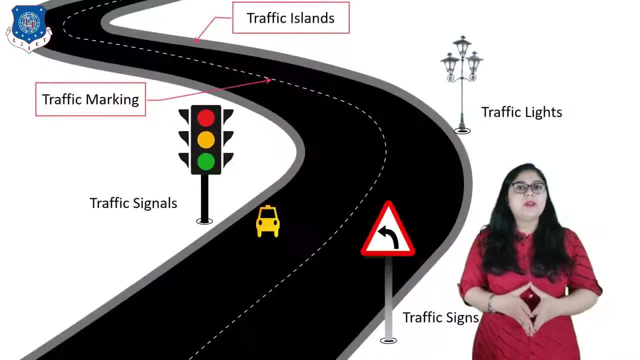 Now let's move to the next traffic control device: traffic lights. It is raised source of light on the edge of a road, which is often mounted on a lamp column or pole, either on the side of the road or within the median, or suspended on a wire above the road. 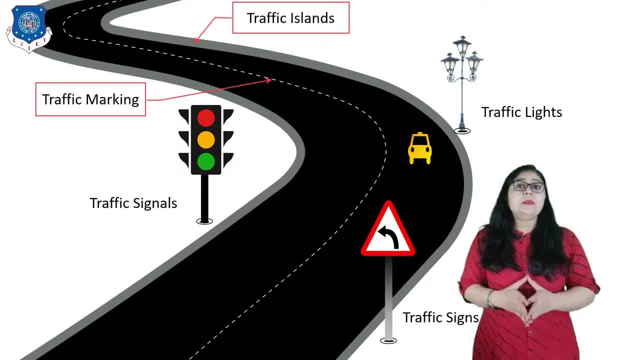 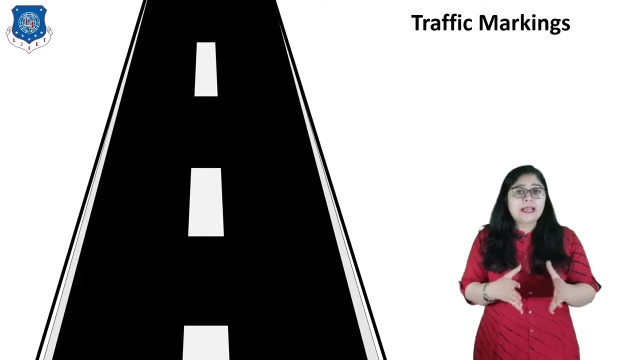 to provide illumination. Straight lighting can provide safety benefits at mid-block and intersection locations and can also improve safety for pedestrians, particularly at crossing roads. Now let's move to the next traffic control devices, which is traffic markings. They are made of lines, patterns, words, symbols or reflectors. 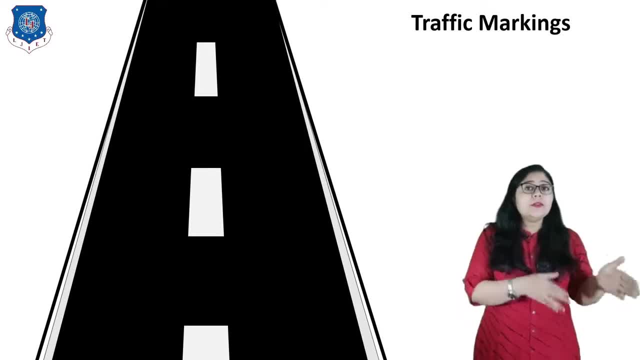 on pavement, Curb, divider or on the fixed objects. They are made using paints in contrast color and brightness. There are a number of types of road markings. Let's discuss all in detail. First type is pavement marking As shown on the screen: white strips in the middle of the road, pavement. 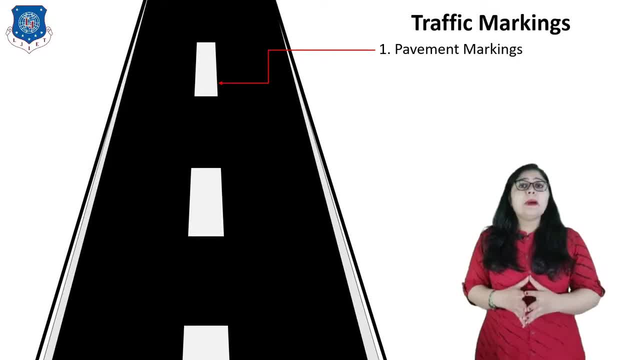 is known as pavement marking. This strip can be marked differently for different purposes, Like here: it is marked as dotted line, which indicate one can change the lane, While a solid line indicates one cannot change the lane or overtaking the vehicles. It helps in smooth and harmonious flow of traffic along guided lanes. 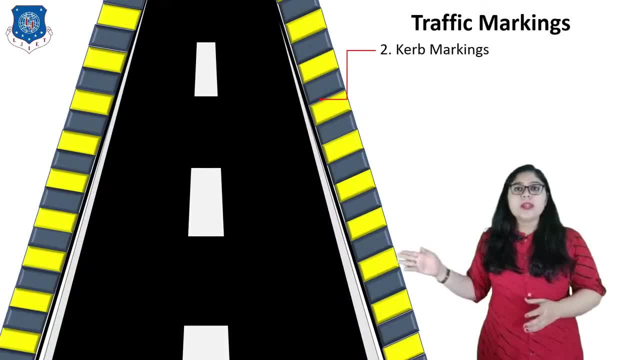 Next type is curb marking. Here you can see black and yellow color strip which is raised portion at the edge of the road. They are painted with either alternative black and white strips too. They divide pedestrian walkway and the roadway. It helps to guide rainwater on the roadway to the drainage line. 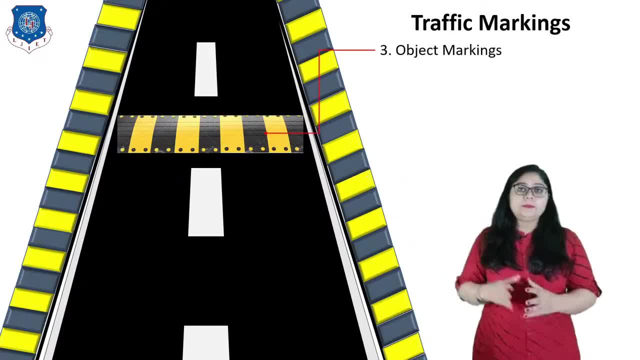 Now next type is object marking. Sometimes objects adjacent to the carriageway may pose some obstruction to the flow of traffic, Objects such as subway piers and abutments or the culvert's headwalls, small temples or tree, etc. 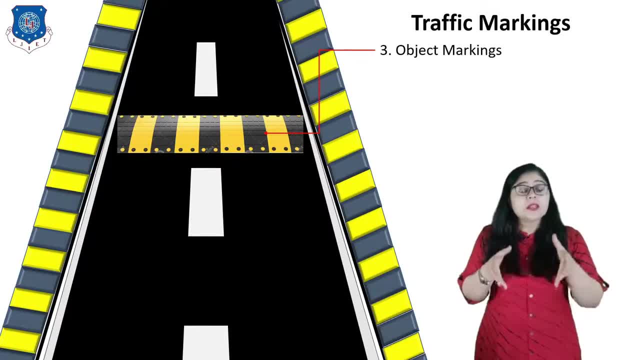 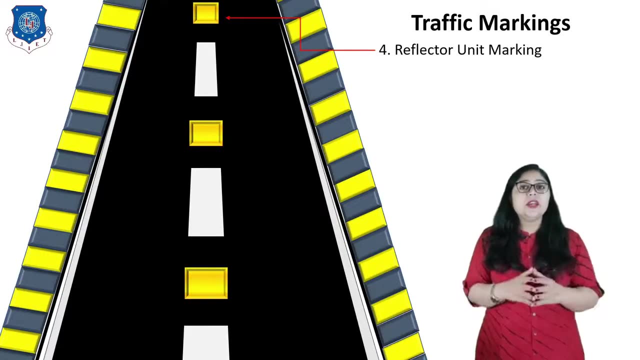 are some example for such obstructions. These cause serious hazard to the flow of traffic and must be marked to reduce accident rate. Now next type is reflector unit marking. It is a safety device used on roads which reflect with light at night. They are made of plastic, ceramic, thermoplastic paints, etc. 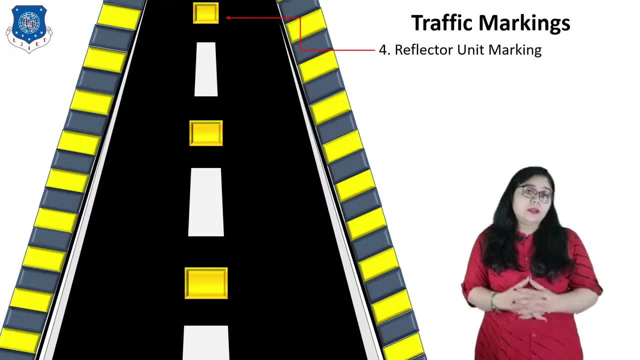 It is available in different shape and color. Mainly placed on the changing line of the lanes and the edges of pavement, It helps to identify boundary of lanes while night driving. Now next type is road delineators. As shown on screen, delineators are tall pylons similar to traffic cones. 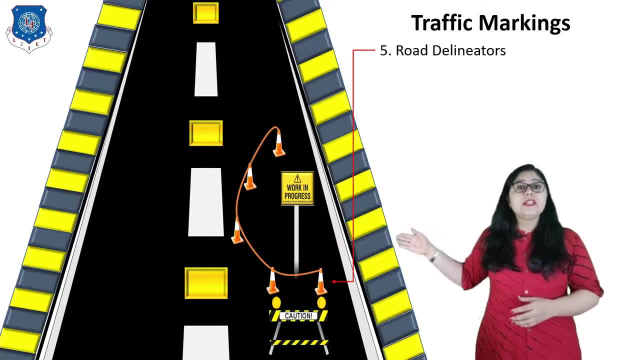 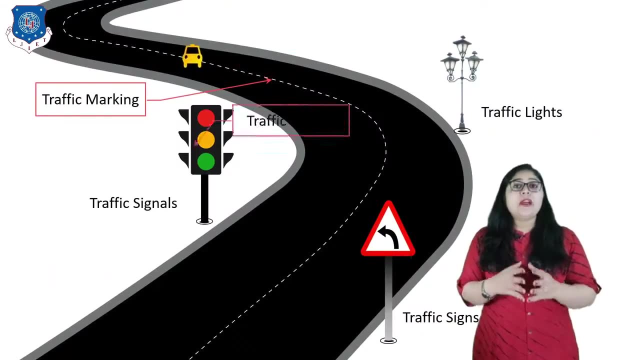 mounted on the road surface or along the edge of a road. They are used to channelize the traffic. They are usually seen on dividers of the bridges and maintenance work. Now let us discuss traffic islands. So traffic islands are raised area constructed within the roadway. 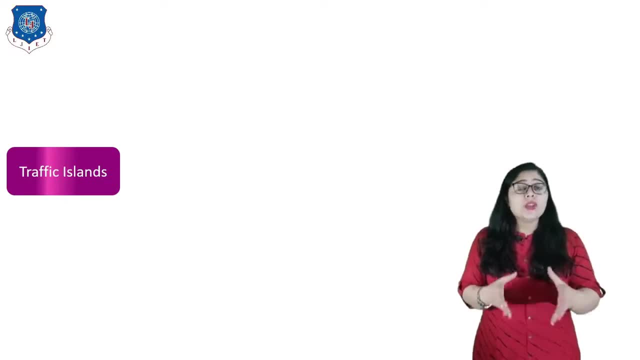 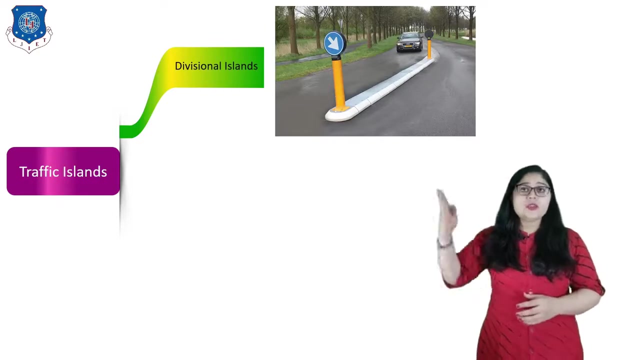 to establish physical channels through which the vehicular traffic may be guided. This can be classified into four types based on the functions. First type is divisional island. It is also called as divider. As shown in the figure, they are intended to separate opposite flow of traffic. 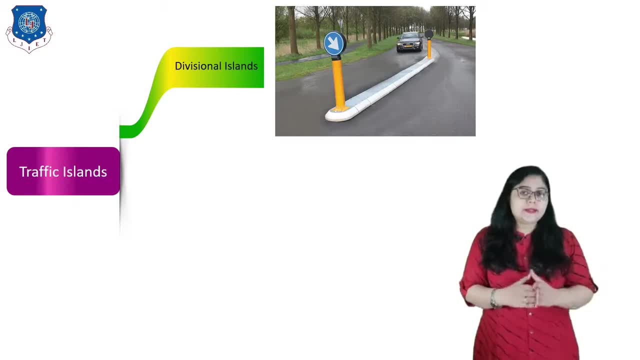 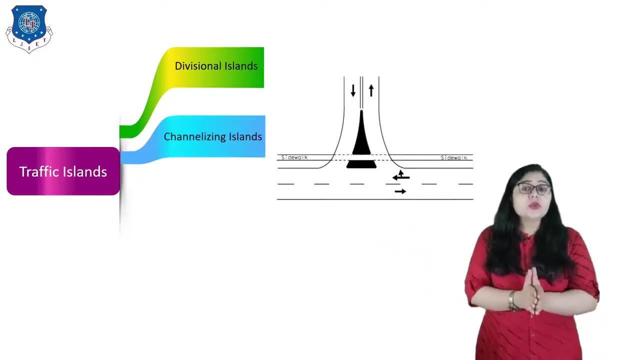 on a highway with four or more lanes, By thus dividing the highway into one way roadway, so that the head on collision can be eliminated. Next is the channelizing island. They are used to guide the traffic into proper channel through the intersection area. It is the separation or regulation of conflicting traffic movements. 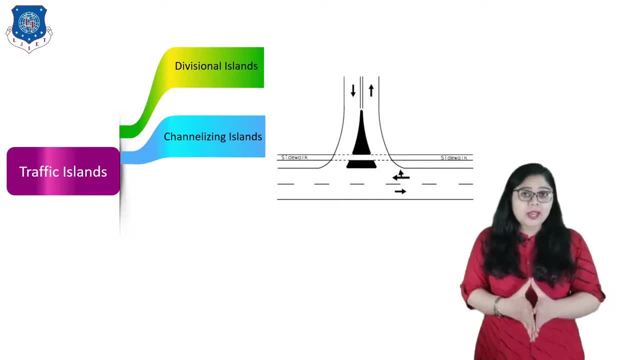 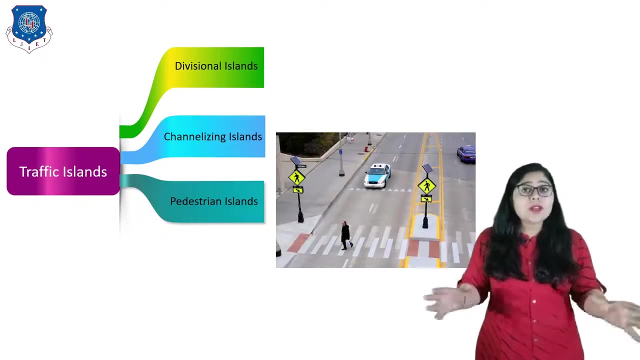 into definite path of travel by traffic islands or pavement marking to facilitate the safe and orderly movements of both vehicles as well as pedestrians. Next is pedestrian island. It is a small section of pavement or sidewalk completely surrounded by asphalt or other road materials, where pedestrian can stop before finishing crossing a road. 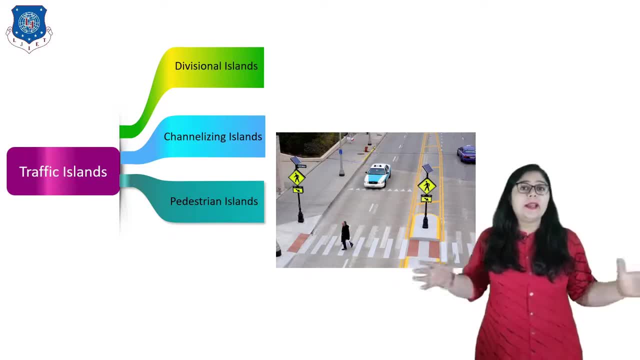 It is typically used when a street is wide, as the pedestrian crossing can be too long for some individual to cross in one traffic light signal. They may also be seen on road with higher speed limits. It reduces the exposure time experienced by a pedestrian in the intersections. 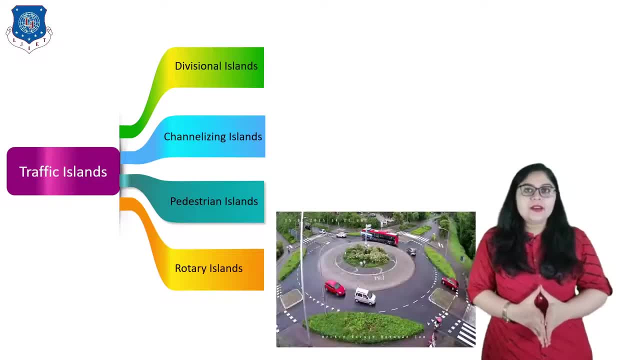 Last is rotary islands. The raised platform of suitable islands and other shapes built on the road intersections are called traffic islands or rotary islands. The main object of providing a rotary are to eliminate the necessity of topping, even for crossing streams of vehicles, and to reduce the area of conflict. 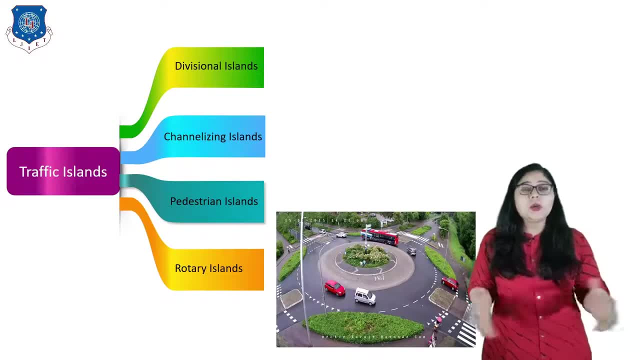 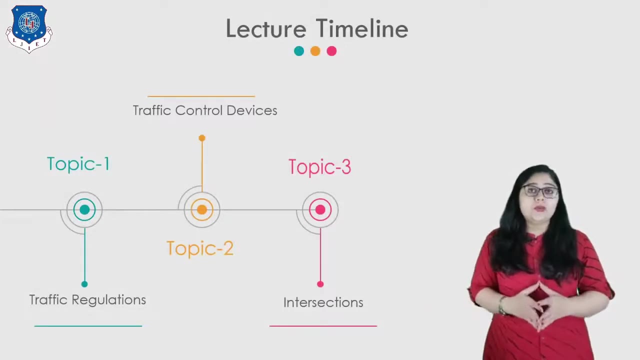 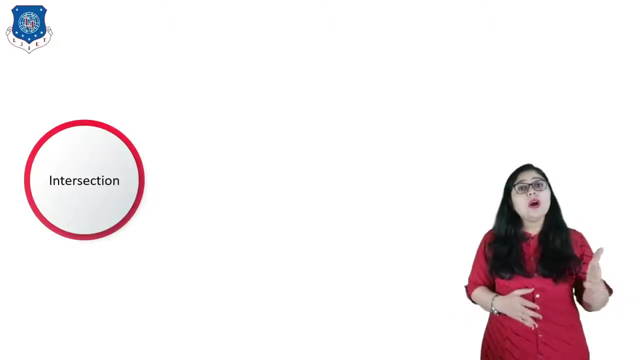 The crossing of vehicles is avoided by allowing the vehicles to merge into the streams around the rotary and then to diverge out to the desired radiating road. Now let's discuss our last topic for today's lecture, which is intersections. So an intersection is defined as the general area where two or more highway joint or cross. 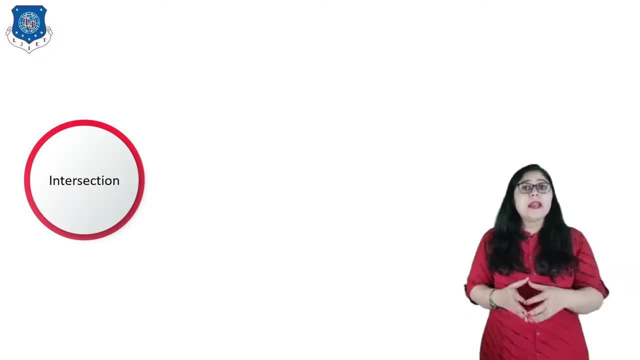 within which are included the roadways and roadside facilities for traffic movement. in that area, The efficiency, safety, speed, cost of operation and capacity of road system very much depend on the intersection design. Various forms of intersections are like T, Y, multiple and cross. 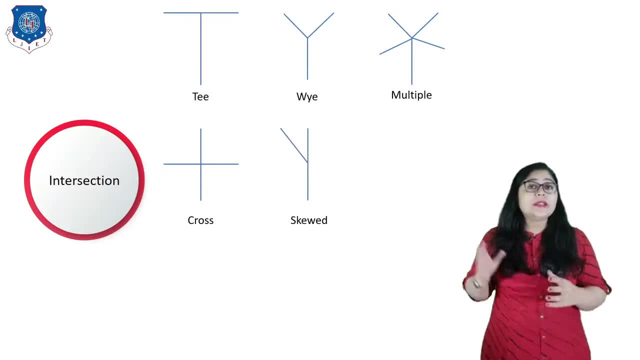 While in skewed one inclined roads is connected with main roads. Here skewed cross is combination of cross and skewed. Next is staggered, which is different than cross intersection, As in cross roads connected to one point, while in staggered it is not connected at one point as it is a staggered. 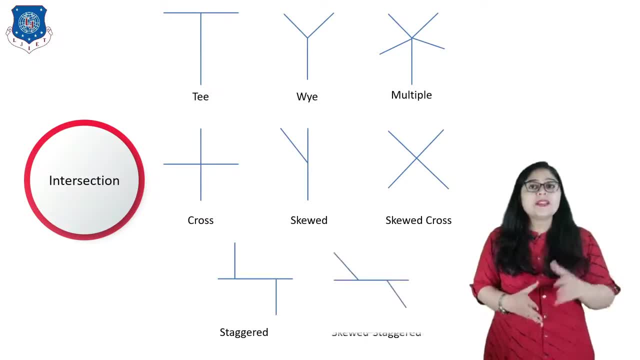 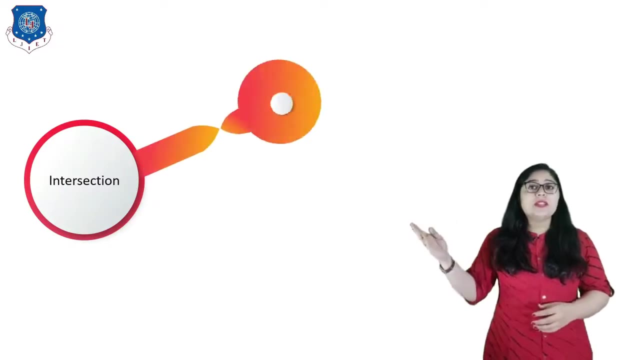 it means in uneven manner. Last is skewed, staggered, which is again a combination of staggered and skewed. Now let's move to the classification of intersection. It is classified into two broad groups: First is at grade and second is grade separated intersection. 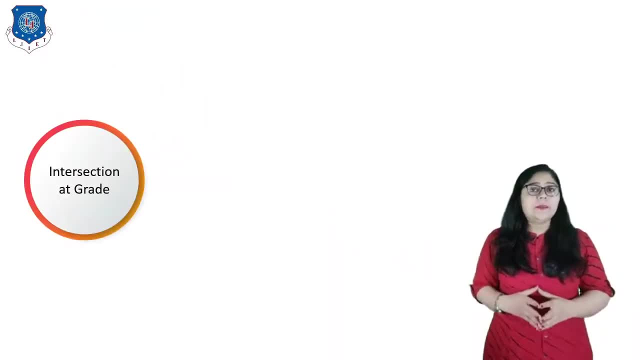 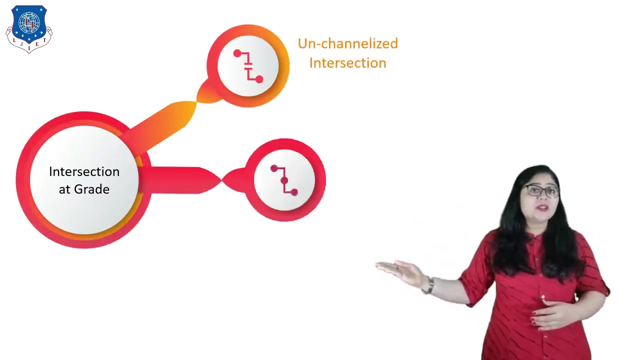 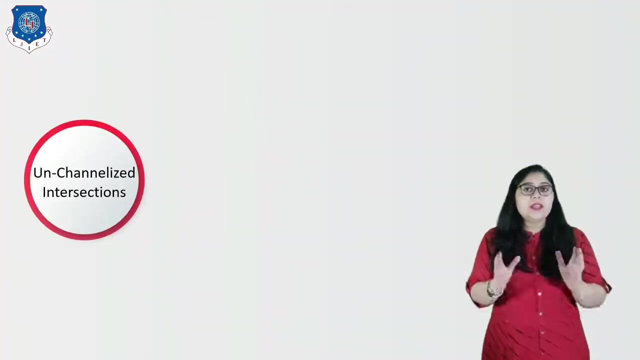 First we will discuss intersection at grade. In this all roads meet about the same level. These intersections can be further classified into three types, like un-channelized intersection, channelized intersection and lastly the rotary intersection. First is un-channelized intersection. In this type of intersection there is no provision of traffic island. 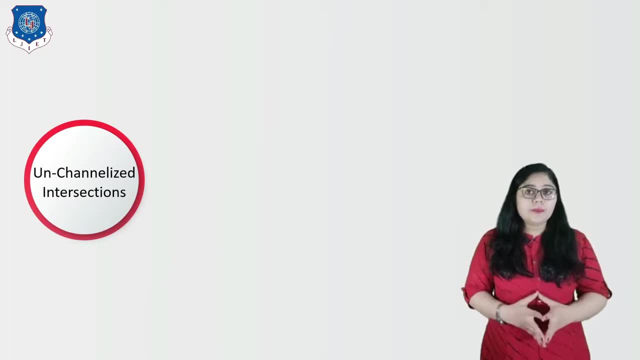 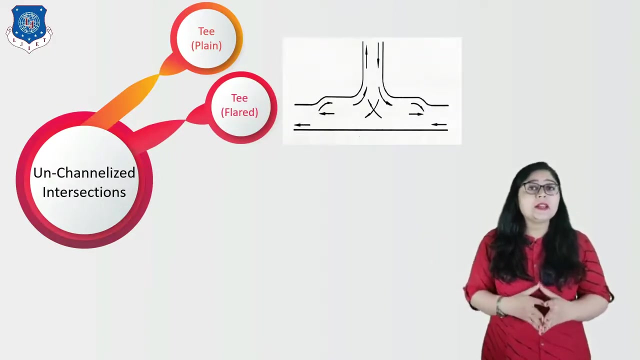 or divider to channelize the traffic flow. Let's see example of un-channelized intersection. First is T-plane intersection. Second is T-flat intersection. Here in flat, at the intersection, the width of road is increased for less congestion of traffic. And the last is cross-plane intersection. 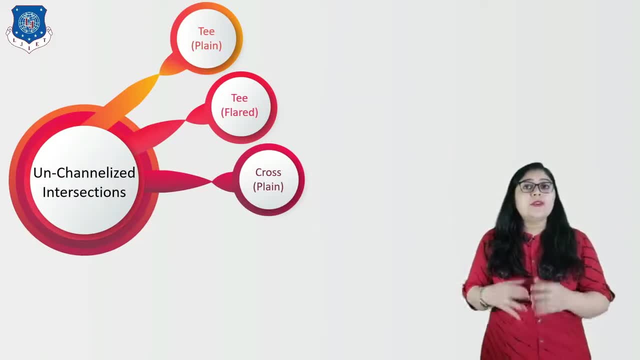 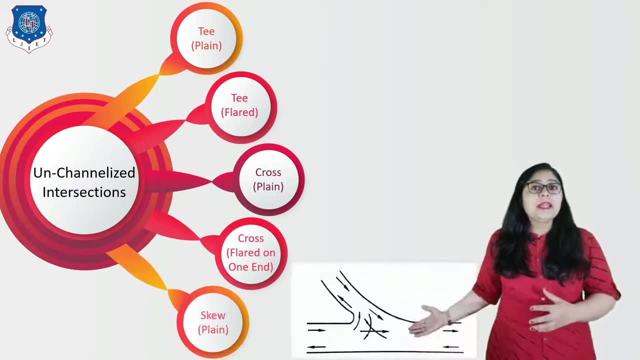 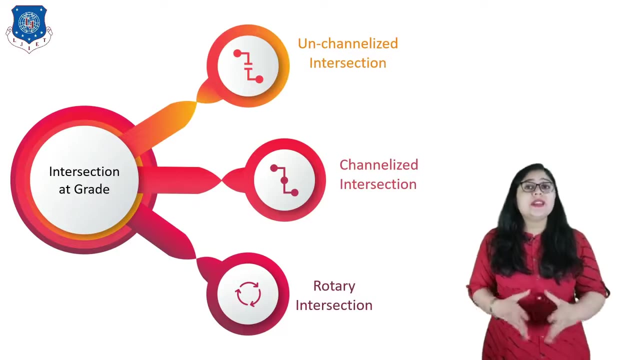 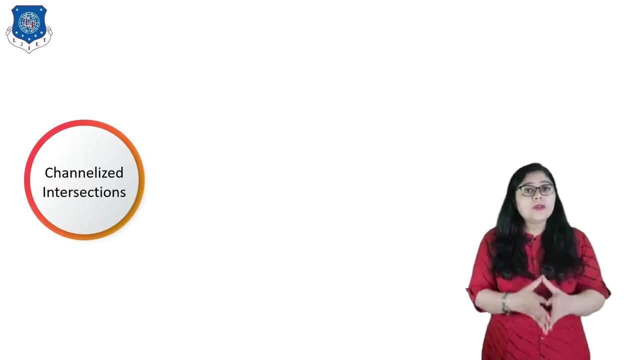 And fourth is cross-flood intersection And lastly, the skew-plane intersection. Now let's move to the second type of intersection at grade, which is channelized intersection. In this type of intersection, traffic island or divider are provided to channelize the flow. 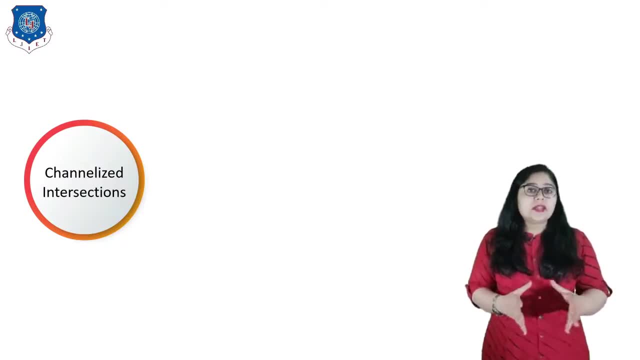 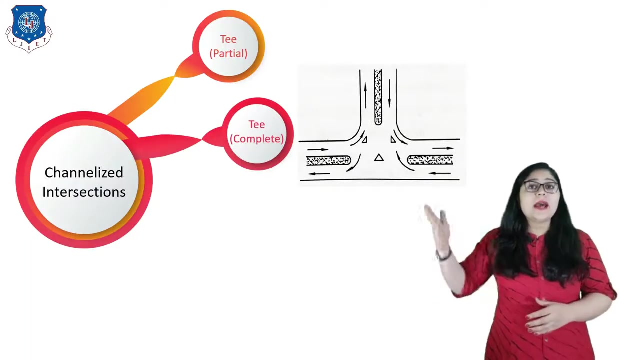 Let's see example of channelized intersection here. First is T-partial channelized intersection in which island or divider are provided only on the main road. you can clearly shown on screen Now. second is T-complete channelized intersection in which all connecting roads are having the island or divider. 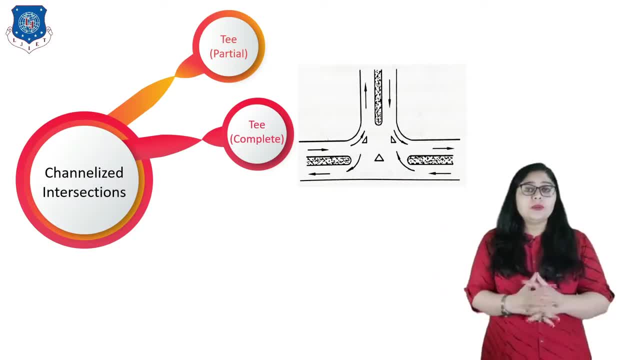 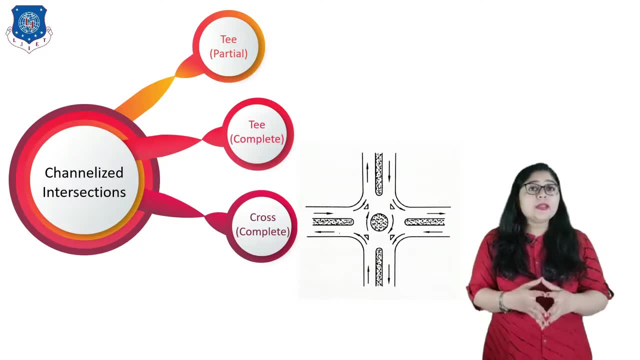 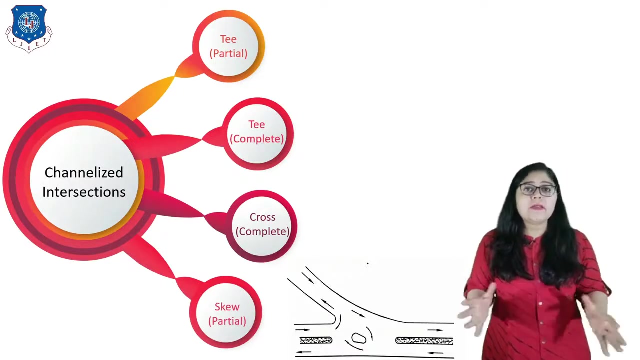 for purpose of traffic flow. Next is cross-complete channelization. As you can see on figure, all four connecting roads are having islands And the last is Q-partial channelization Because of part-partial inclined road is not having island, only major road are having islands. 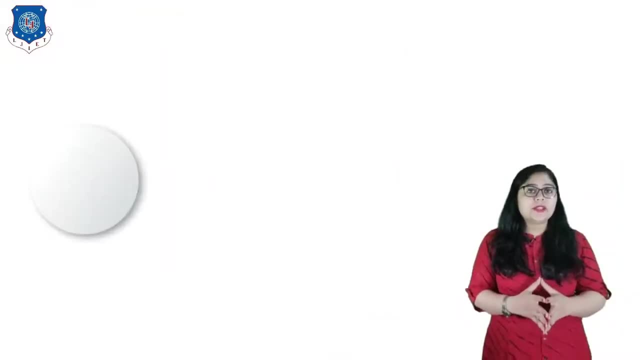 Now let's move to the third type of intersection at grade, which is rotary intersection. A rotary intersection is a specialized form of intersection at grade in which the traffic moves in one direction around a central island. For keep to the left rule, the vehicle approaching the intersections are forced to move around the central islands. 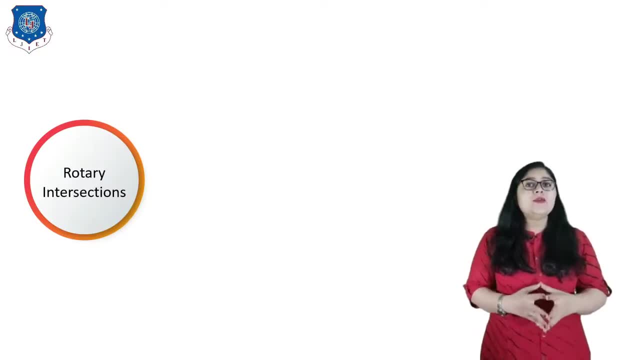 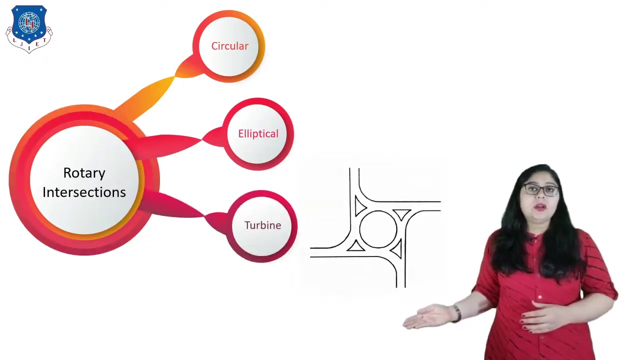 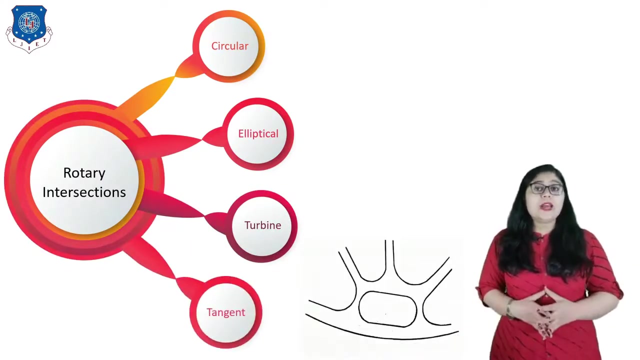 in an orderly manner and weave out of the rotary into their respective desired directions. Let's discuss the various types of rotary intersections. First is circular, Second is elliptical, Third is turbine type And last is tangent intersection. So these all four types are based on their shape. 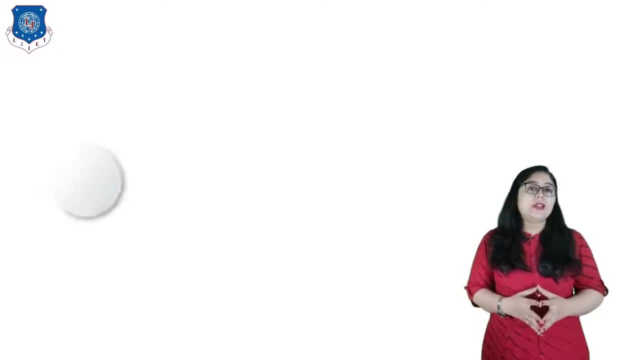 Now let's move into the second type of intersection, which is grade separated intersection. In this type of intersections, intersecting road are separated by difference in level, thus eliminating the crossing problem. This type of intersection cause least delay and hazard to the crossing traffic. It increases traffic safety and gives efficient operation. 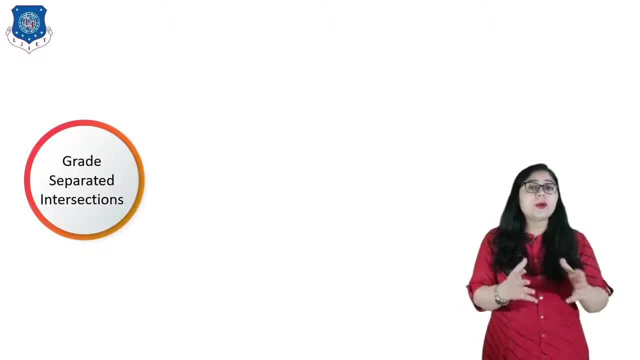 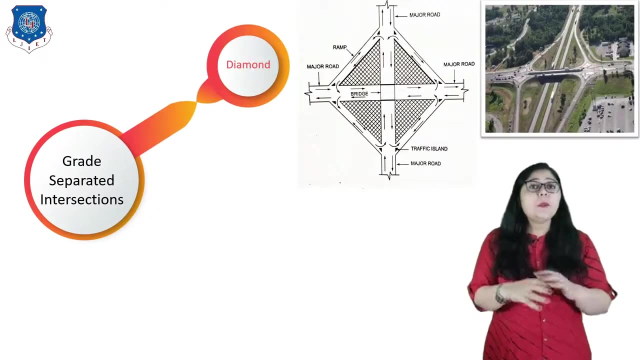 of traffic flow. Let's discuss the example of grade separated intersections. First is diamond interchange, which is a popular form in urban locations where major and minor roads are crossing at different levels. as shown on screen, It is designed for relatively narrow right of way of major roads. 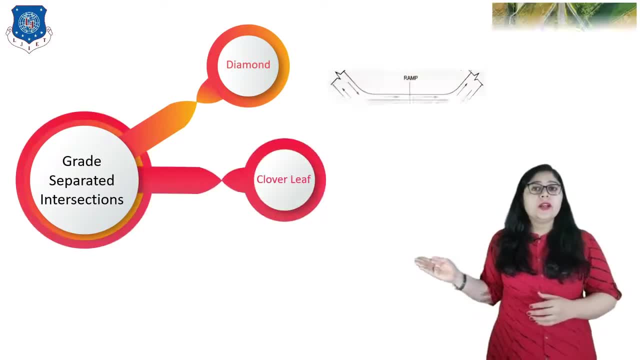 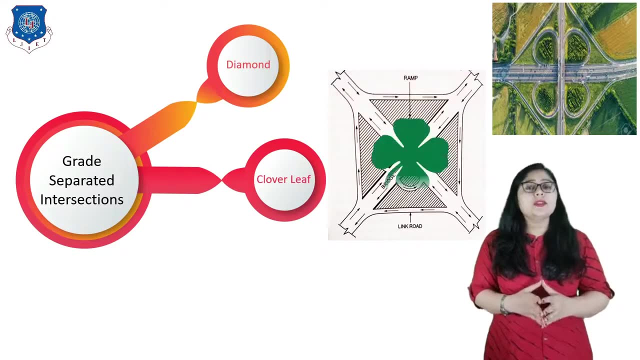 Second is clove leaf interchange. Its name comes from one leaf having same shape, which is shown on screen. This is a four leg interchange with a single structure. It is popular and used when two high volume and high speed roads are intersecting with each other.